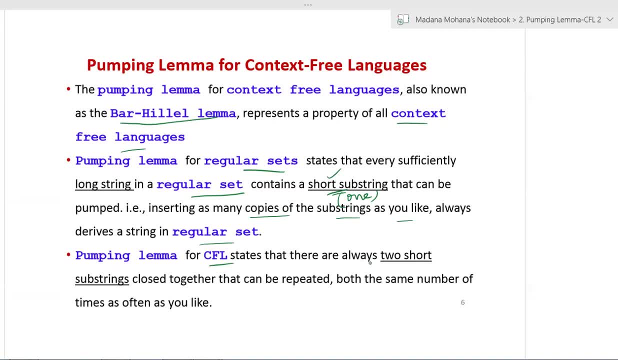 Whereas pumping lemma for context free languages is a part of the structure of the structure, context-free languages states that there are always two short substrings close together that can be repeated both the same number of times, as often as you like. So here two substrings can be repeated with same number of time in pumping lemma for context-free. 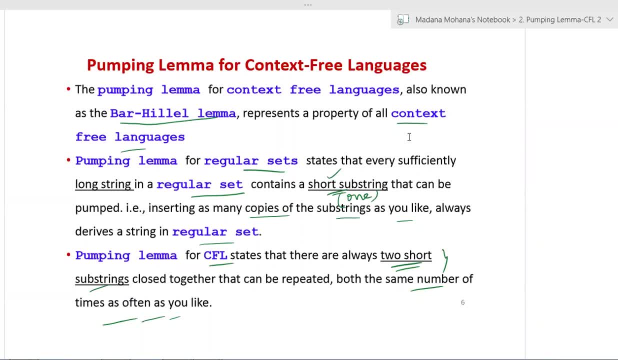 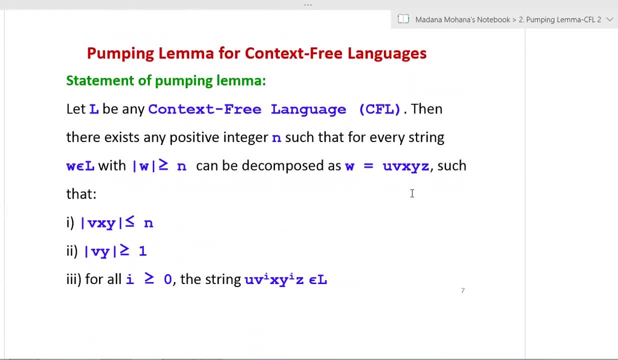 languages whereas regular languages. pumping lemma, only one substring. that is the only difference remaining. all are same. Then let us see the statement of pumping lemma. So let L be any context-free language. then there exists any positive integer, say small n, such that for every string W belongs to L, W is the string where the length of the string 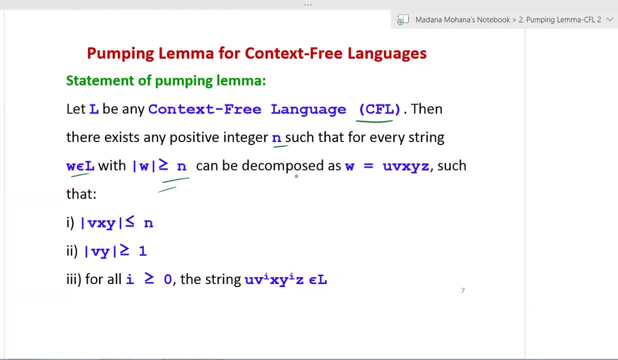 that is, mod W is greater than or equal to n, can be decomposed as u, v, x, y, z. Here you can see that the length of the string is greater than or equal to n. So here you can see, whereas in regular language, pumping lemma, the string is decomposed into only x, y, z. This 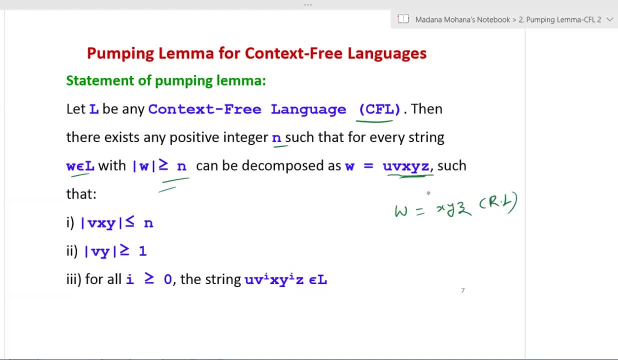 is for regular language pumping lemma Now, whereas here five substrings, that is, u, v, x, y, z. So in regular language pumping lemma x, y, power, i, z, only this can be pumped, y, power, i. But whereas in regular language pumping lemma x, y, power, i, z, only this can be pumped. 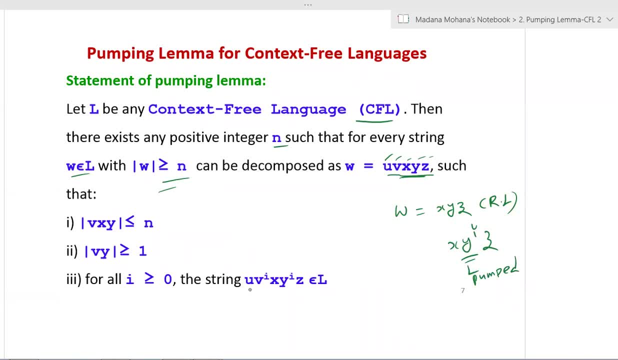 y power i. In context-free language, pumping lemma. here you can see two substrings, that is, v power i, y power i. So two can be pumped at the same time with the same power value. That is the difference remaining. all are same. Now you can see the string W can be decomposed. 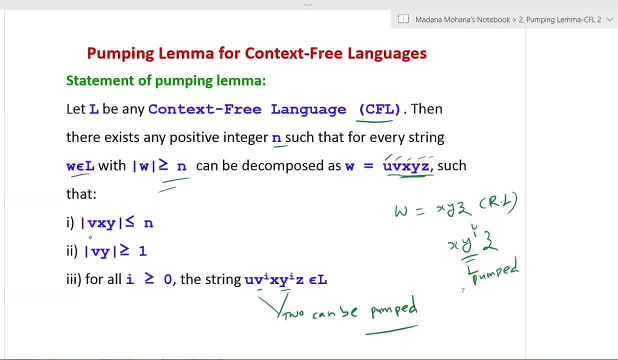 as u v x y z, such that now the first condition, mod v x y, that is, the length of v x y z- is less than or equal to n. Then mod v y: these two can be pumped, repeated the same number of times. That is the length of mod v y, always greater than or equal to one. Then the third: 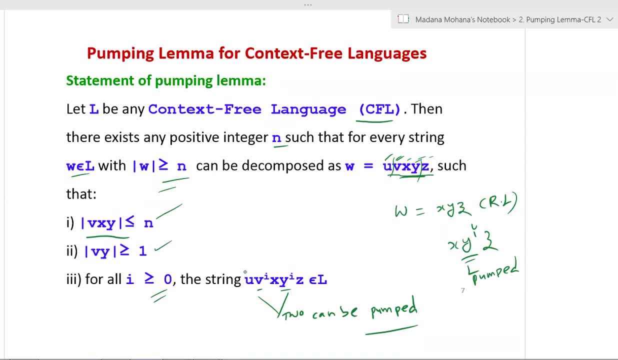 condition for all i greater than or equal to zero, the substring u, v power, i, x, y, power, i, z. for all values of i. i value zero to n. If you can substitute i value as zero, then u x, z. if it is belongs to l, the resultant string. if it is belongs to l, then it satisfies. 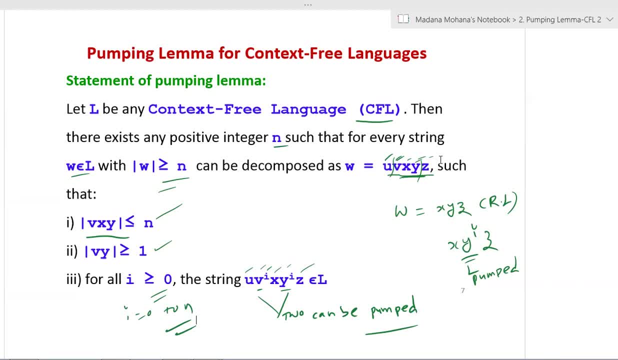 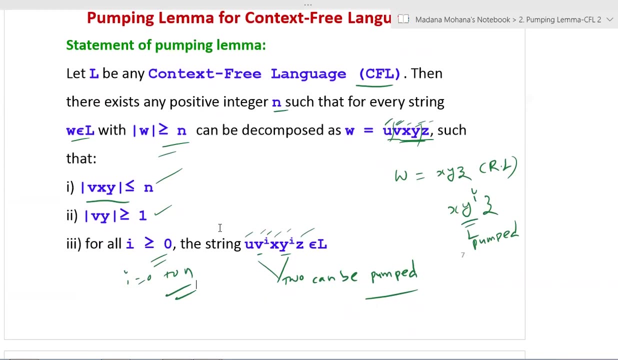 the condition of pumping. i mean pumping lemma. Therefore the language is context-free language for any value of i. if it is not belongs to l, then it violates the pumping lemma. then you can say l is not context-free. The same process as a regular such, but only decomposing. 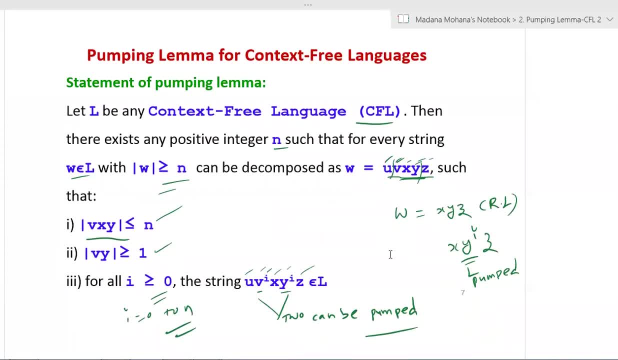 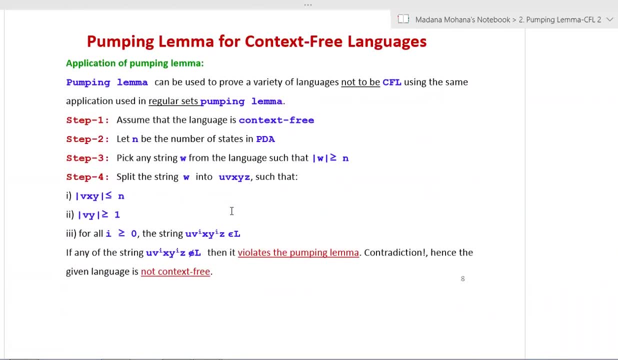 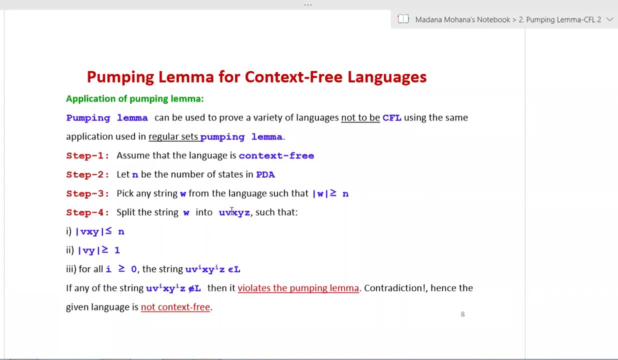 of the string into three substrings. there here five substrings, Here two substrings. can be repeated same number of times. These are all the differences. They are coming to. application of pumping lemma for context-free languages. The same steps here also will use. 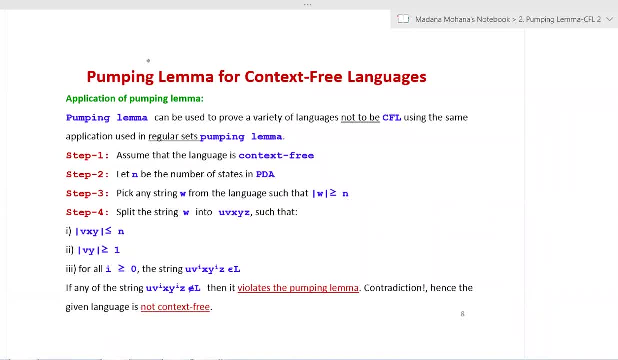 as it is in regular languages: pumping lemma. So pumping lemma can be used to prove a variety of languages not to be context-free language. Using the same application used in regular sets- pumping lemma- Step one, as usual, assume that the language is not context-free, Whereas in regular language we assumed the language. 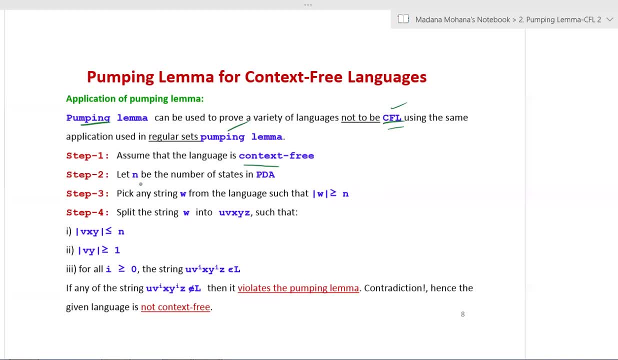 is not regular but yet context-free. that is the difference. Then let n be the number of states in PDA. Why? because context-free languages are accepted by PDA. That is why, here, we have considered the acceptor PDA, Whereas regular languages it is accepted by finite automata. 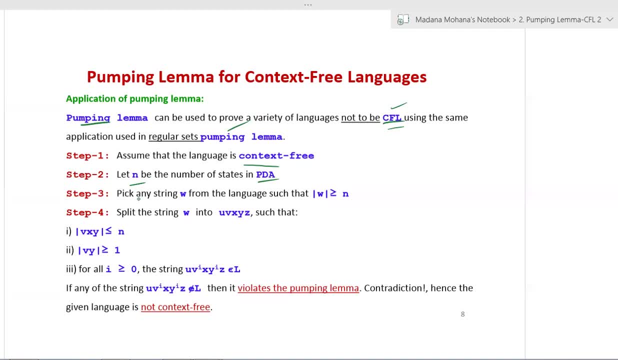 So there the states of finite automata we have to consider. that is the difference. So that is the difference. Now, pick any string w from the language such that mod w greater than or equal to n. Then you have to split the string w into five substrings, as u, v, x. 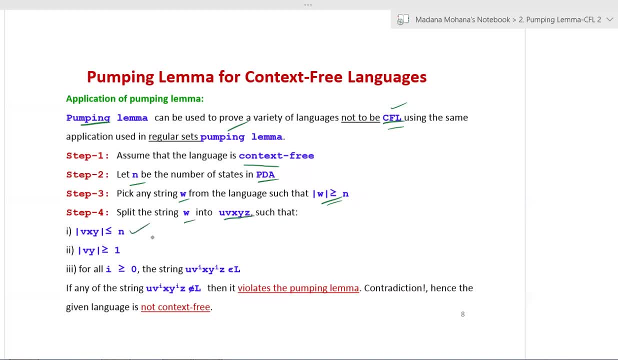 y z, such that mod v x y less than or equal to n, Then mod v y greater than or equal to 1.. Then, for all i greater than or equal to 0, the string u v x, y, power i z, if it is, belongs. 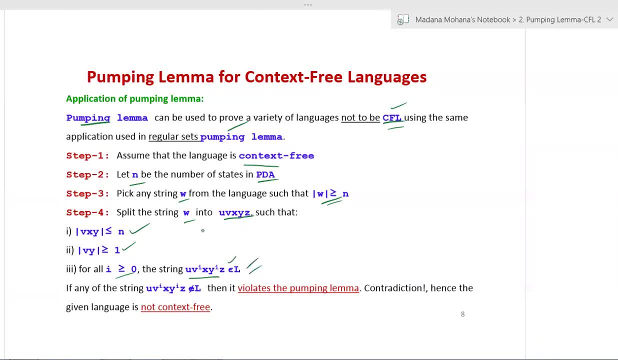 to l, Then we can say: the language is context-free. Suppose: if any of the string u, v, power, i, x, y, power, i, z not belongs to l, Then it violates the condition of pumping lemma. Then, contradiction, our assumption is false, Hence the given language. 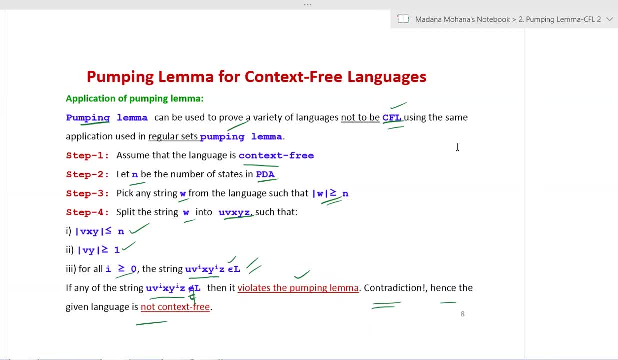 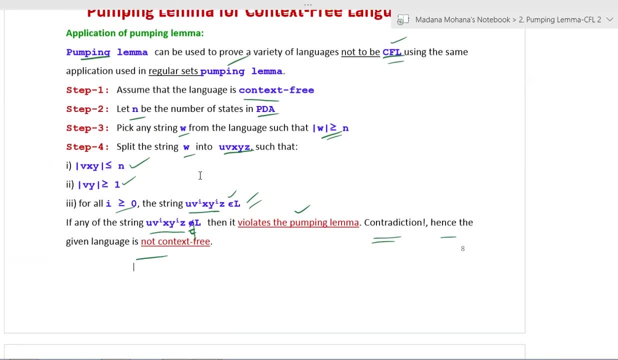 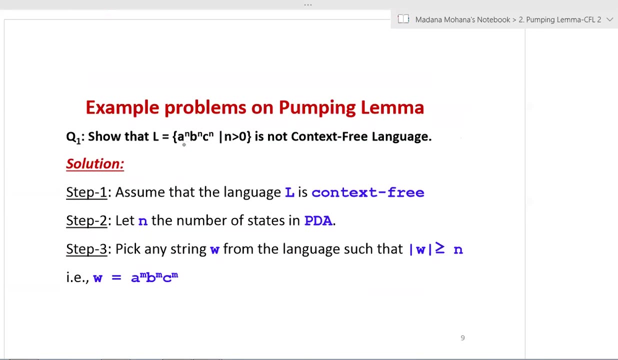 is not context-free. So, like that, we have to prove a language which is not context-free using the application of pumping lemma for context-free languages. Now let us see one example. So the question is given like this: Show that l equal to a power n b power n, c power n, such 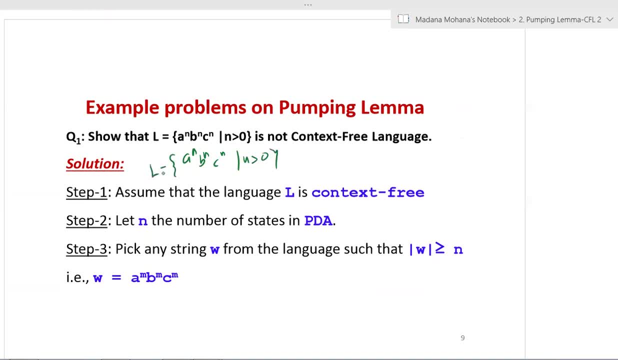 that n greater than 0 is not context-free language. Here you can see In the given question they won't mention pumping lemma. By seeing this question itself you can identify the pumping lemma If the question is a language which is not regular language. 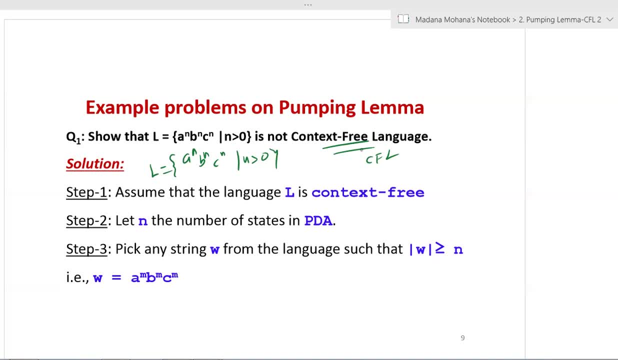 You can apply pumping lemma for regular sets or regular language. A question is like this: A language is not context-free, Then you can apply the pumping lemma for context-free languages. Like that. you can identify. So now as well the application. what are the steps we mentioned? 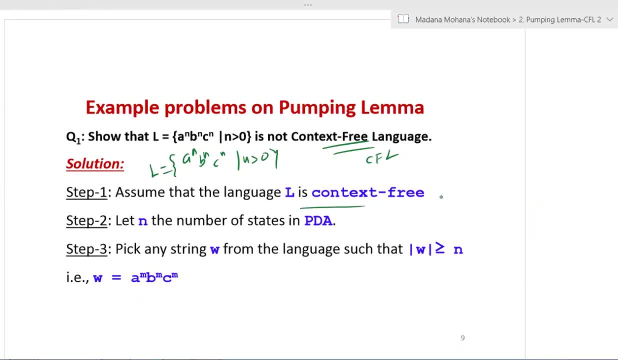 Same steps. you can use Step one. assume that the given language is context-free. Second step: let us take n, the number of states in PDA, Then pick any string w from the language such that mod w greater than or equal to n, That is, let us take any substing from l. 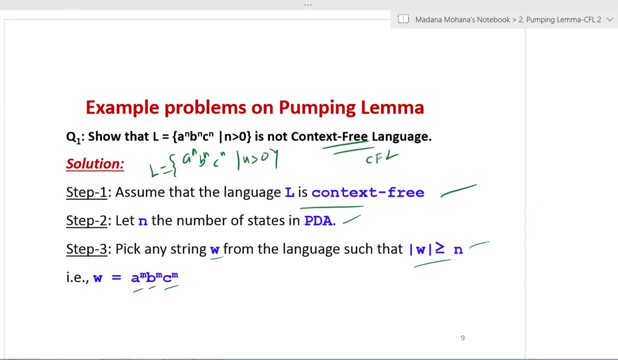 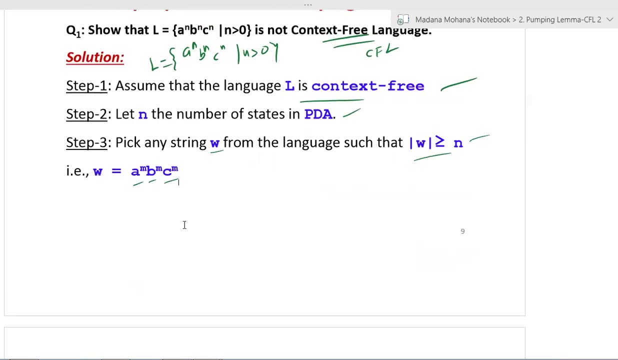 Here we assumed as a power n, b, power n, c, power n, Where the original is with power n. We have taken some other power, But same power for all: a, b, c. So the nature of this language is number of a's, followed by number of b's, followed by number of c's. Now, next step, we 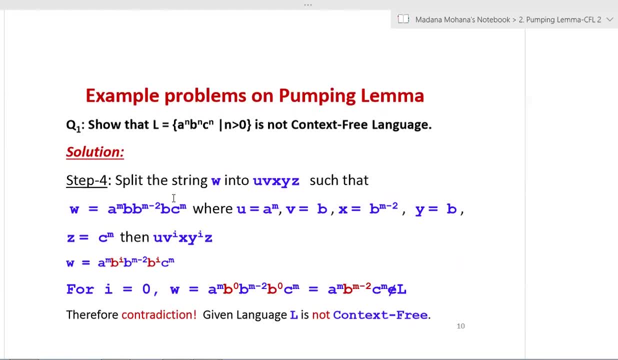 thing w into five parts as u v, x, y z format, so w into u v x, y z, such that whenever you are splitting it should satisfy the above conditions. that is, mod v, x, y less than or equal to 1, mod v by greater than or equal to 1, then for all i greater than or equal to 0. u v, power i, x, y, power i z belongs to. 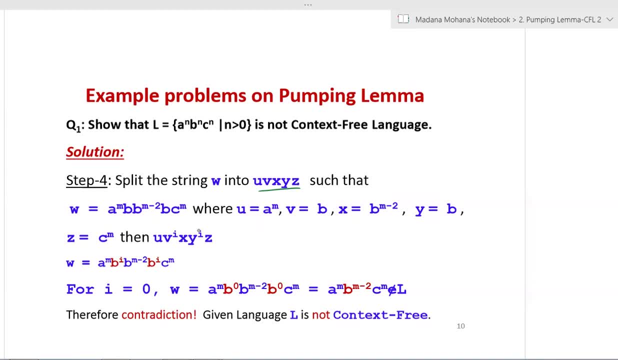 l. if so, the language is context free, otherwise it is not context free. so now that w can be decomposed as, let us see here: a power m, now c power m as it is now b is decomposed with three substrings that like b, b power m minus 2, b again. if you can simplify this, one b power. 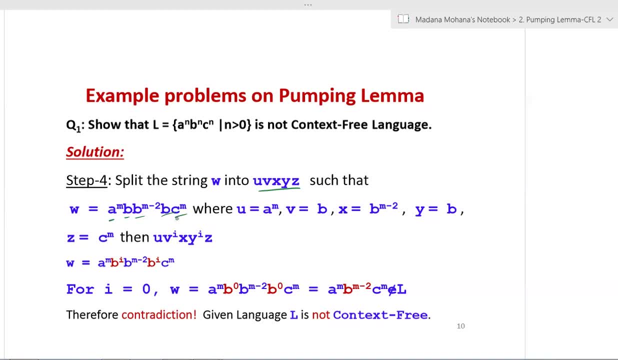 1 plus m minus 2 plus 1, you will get b power m only. there is no chain. even you can split c power m also, a power m also. you can split c power m also, a power m also, but you have to satisfy the conditions. so now in this split you can convert into u, v, x, y, z format. 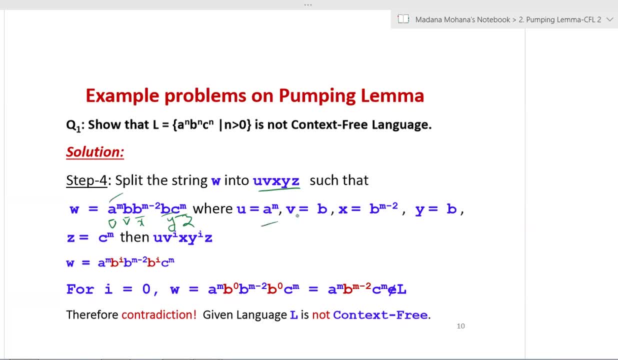 now where u is a power m here, v is b, then x is b power m minus 2, then y is again b, then c is i mean z is c power m. so then you can find out this value: u, v, power i, x, y power i, z. so now u means a power m, v means b power i, then x means b power m minus 2. 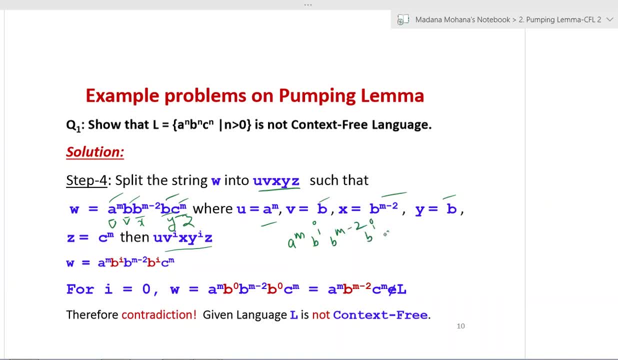 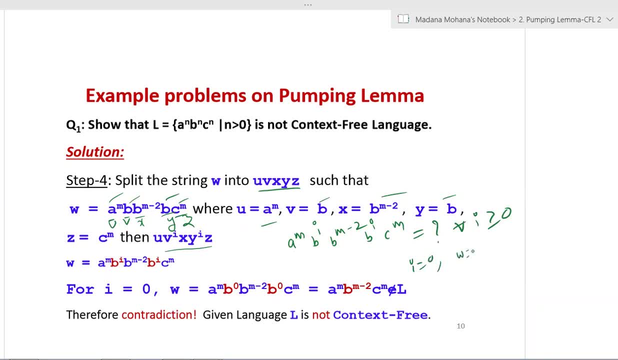 for all values of i. if it is belongs to l, then only it satisfies the condition of pumping level. for i equal to 0. let us see w equal to a power m, b power 0, b power m. minus 2, b power 0, then c power m. for i equal to 0, let us see w equal to a power m. b power 0. b power 0. b power m minus 2. b power 0, then c power m. for i equal to 0, let us see w equal to a power m. b power 0. b power 0, then c power m. 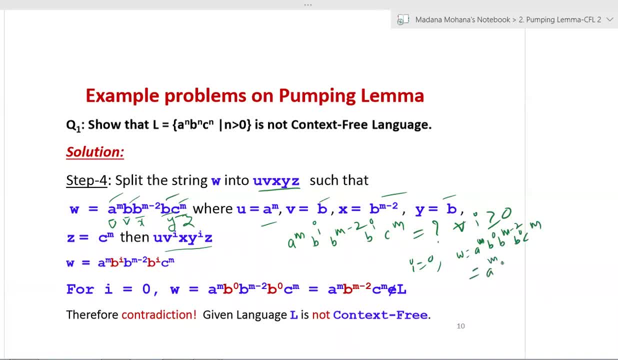 for i equal to 0. let us see w equal to a power m. b power 0, b power 0. then c power m. simplify this one: here you will get a. simplify this one, here you will get a. simplify this one: here you will get a power m. b for 0 means 1, then b power m. power m: b for 0 means 1 then b. power m. power: m: b for 0 means 1 then b. power m minus 2: b for 0 means again 1 then c. minus 2: b for 0 means again 1 then c. 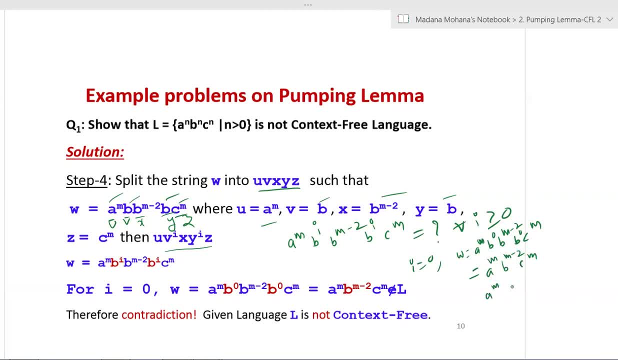 minus 2, b for 0 means again 1, then c: power m. now you can see you are given power m. now you can see you are given power m. now you can see you are given. original language is a power m, b power m. original language is a power m, b, power m. 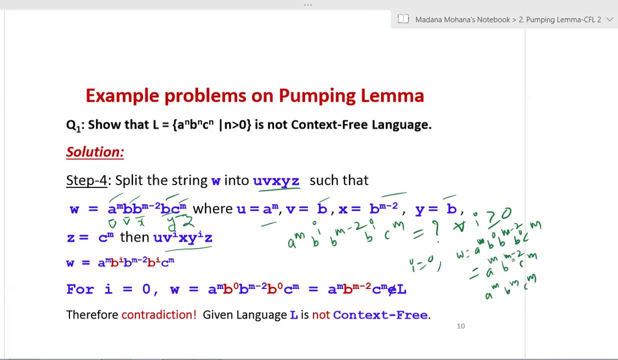 original language is: a power m. b power m, c power out. but here you can see b power, c power out. but here you can see b power, c power out. but here you can see b power. m minus 2 is there. m minus 2 is there. 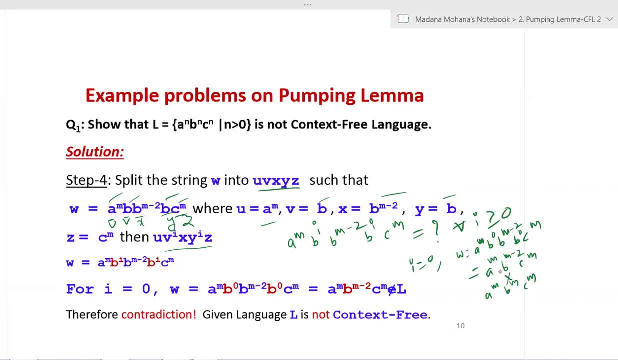 m minus 2, is there? so so? so, two b's are reduced here. this is not. two b's are reduced here. this is not. two b's are reduced here. this is not equal to here. therefore, equal to here, therefore, equal to here, therefore, which is not belongs to l. 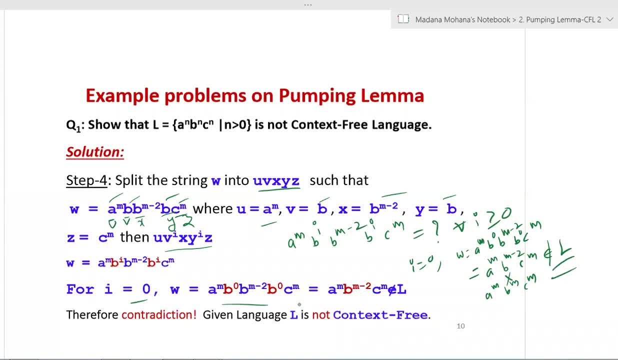 which is not belongs to l which is not belongs to l. now you can see i equal to 0 w equal to now. you can see i equal to 0 w equal to now. you can see i equal to 0 w equal to here. this one so, which is not belongs. 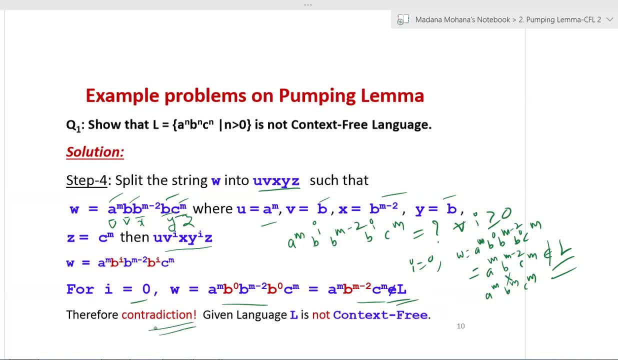 here. this one so which is not belongs here, this one so which is not belongs to here. therefore, contradiction to here. therefore, contradiction to here. therefore contradiction. the condition of pumping lemma application. the condition of pumping lemma application. the condition of pumping lemma application. here you can see, here you can see. 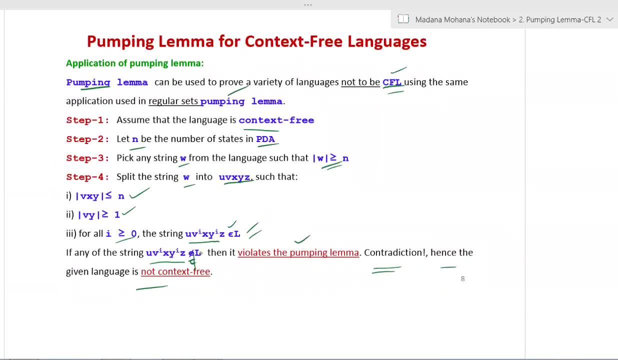 here you can see. so if any string u, v power, x, y power, so if any string u v power, x, y power, so if any string u v power, x, y power, z not belongs to l, then it violates the z not belongs to l, then it violates the. 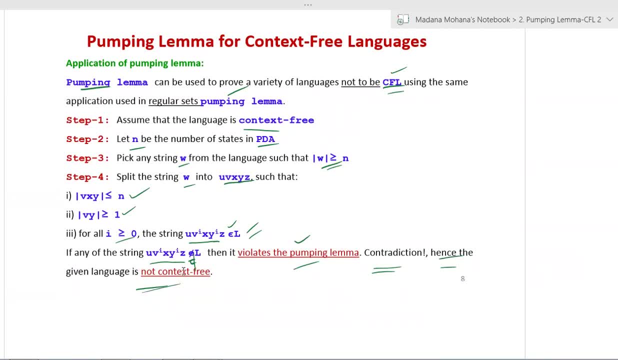 z not belongs to l, then it violates the pumping lemma contradiction, hence the pumping lemma contradiction. hence the pumping lemma contradiction. hence the given language is not context free, so given language is not context free. so given language is not context free. so it's satisfying the violation condition. 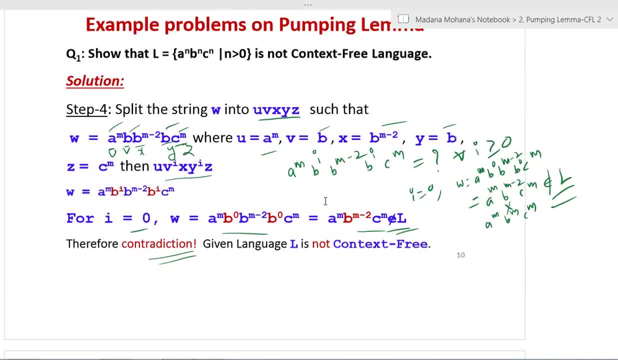 it's satisfying the violation condition. it's satisfying the violation condition. so, therefore, so, therefore, so, therefore, that conclusion, you can write down, that conclusion, you can write down that conclusion. you can write down, therefore, contradiction, here, the given. that conclusion you can write down. therefore, contradiction, here, the given. 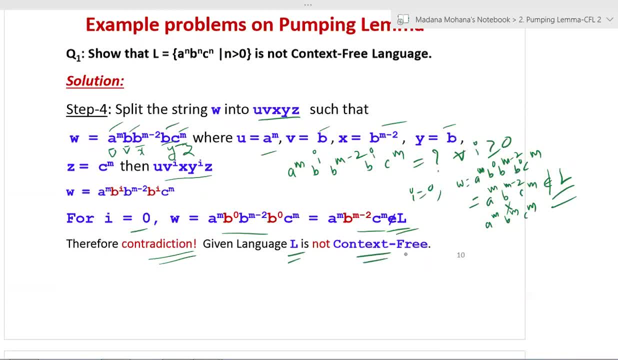 that conclusion you can write down, therefore, contradiction here: the given language, l language, l language l is not context free. suppose if it is is not context free. suppose if it is is not context free. suppose if it is belongs to l, belongs to l belongs to l. then you can check for other value of 5. 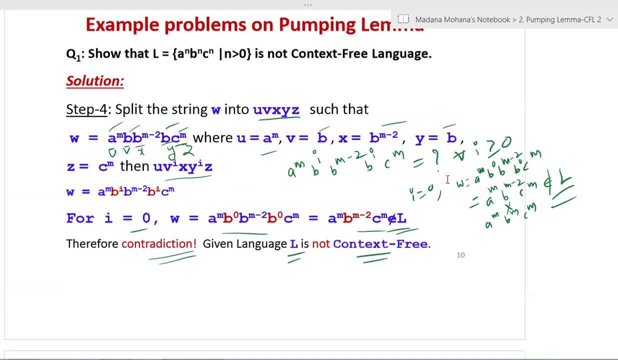 then you can check for other value of 5. then you can check for other value of 5 for all values. it has to satisfy for all values. it has to satisfy for all values. it has to satisfy for violation, even for a single value. it for violation, even for a single value. it. 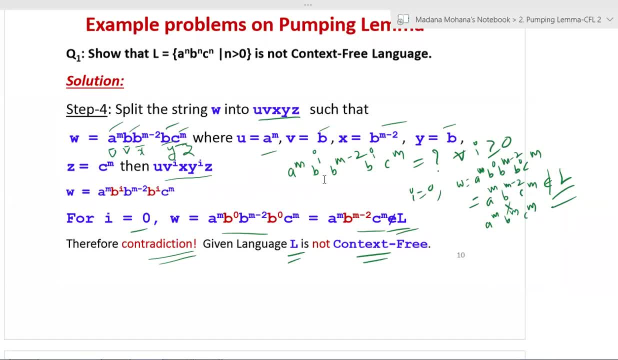 for violation, even for a single value, it violates it, violates it. violates it, then you can say contradiction: it is not, then you can say contradiction. it is not, then you can say contradiction: it is not. context free language like that you can. context free language like that you can. 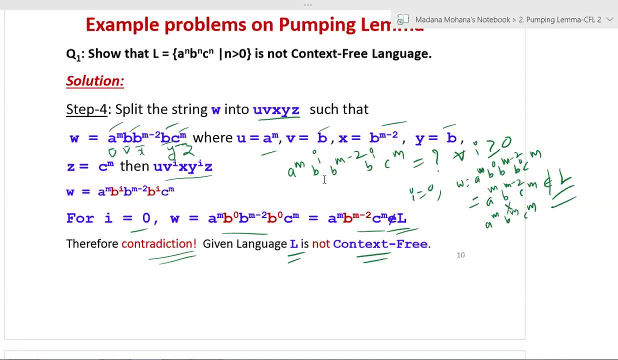 context free language. like that, you can prove any given language which is not prove any given language which is not prove any given language which is not context free. using the pumping lemma for context free. using the pumping lemma for context free. using the pumping lemma for context free languages. 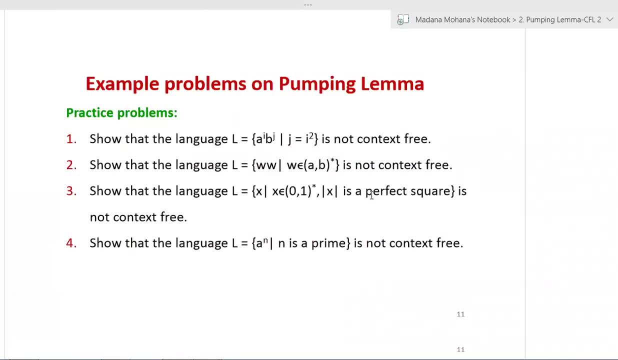 context free languages, context free languages. now, here, some practice problems are given. now, here, some practice problems are given. now, here, some practice problems are given. you can, you can, you can do in the similar manner. so don't do in the similar manner. so don't do in the similar manner, so don't worry about the question, whatever the 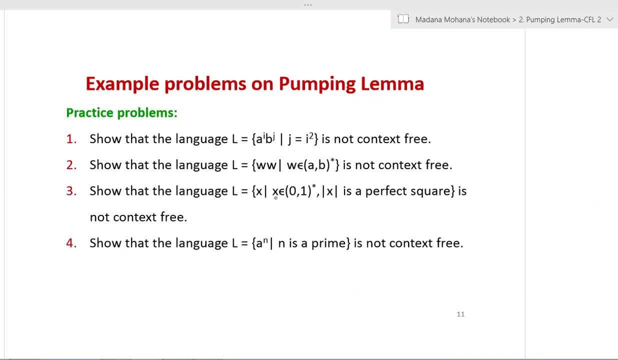 worry about the question, whatever the worry about the question, whatever the given question, given question, given question, by satisfying the conditions. take one by satisfying the conditions. take one by satisfying the conditions. take one string, string, string. that string can be decomposed into u v x. that string can be decomposed into u v x. 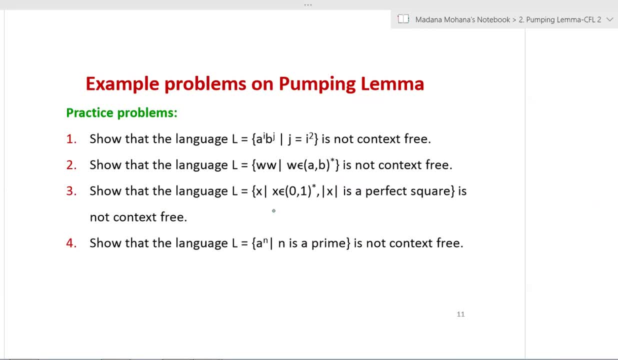 that string can be decomposed into: u v, x, y z format by satisfying the three y z format. by satisfying the three y z format, by satisfying the three conditions of pumping lemma, then the last conditions of pumping lemma, then the last conditions of pumping lemma, then the last condition: u v, power i, x, y, power i z. 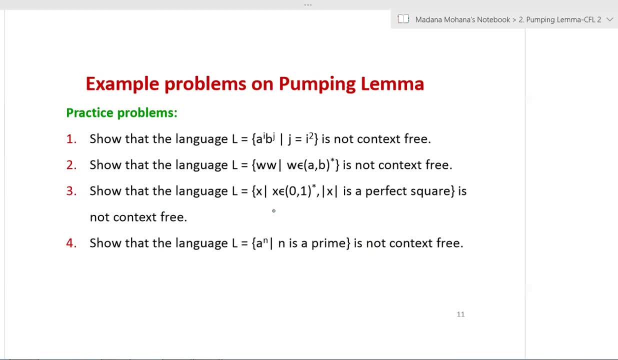 condition u v- power i x y, power i z. condition u v- power i x, y, power i z. for all values of i starting with zero. for all values of i starting with zero. for all values of i starting with zero. you can substitute and check even for. 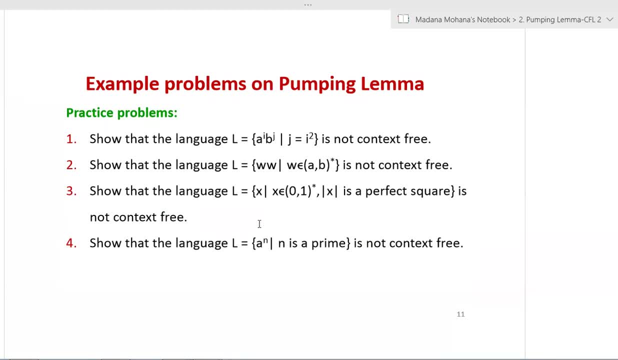 you can substitute and check even for. you can substitute and check even for single value. if anything not belongs to single value, if anything not belongs to single value, if anything not belongs to l, then it violates the condition of l. then it violates the condition of l, then it violates the condition of pumping lemma. then you can say: 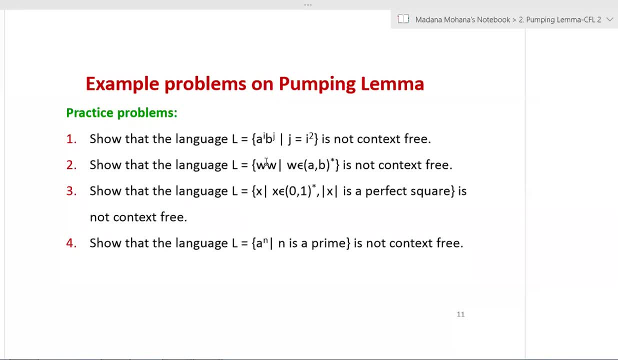 pumping lemma. then you can say: pumping lemma. then you can say: the given context. v is language is not the given context. v is language is not the given context. v is language is not context free. like that you can context free. like that you can context free. like that you can prove a language which is not context free. 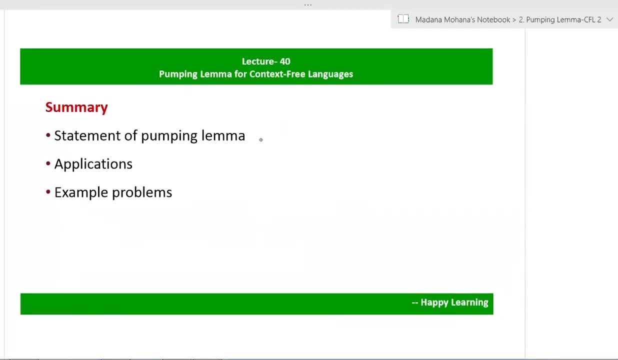 prove a language which is not context free. prove a language which is not context free, then coming to summary, then coming to summary, then coming to summary. so here first we discuss the statement. so here first we discuss the statement. so here first we discuss the statement of the pumping lemma. 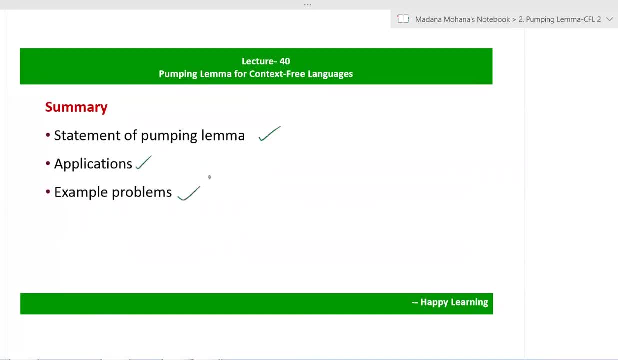 of the pumping lemma, of the pumping lemma, then applications of the pumping lemma, then applications of the pumping lemma, then applications of the pumping lemma. then one example problem is demonstrated. then one example problem is demonstrated. then one example problem is demonstrated, then some practice problems are given. then some practice problems are given. 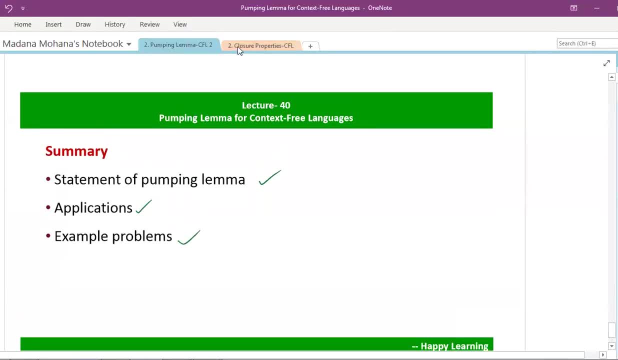 then some practice problems are given. those also you can practice.